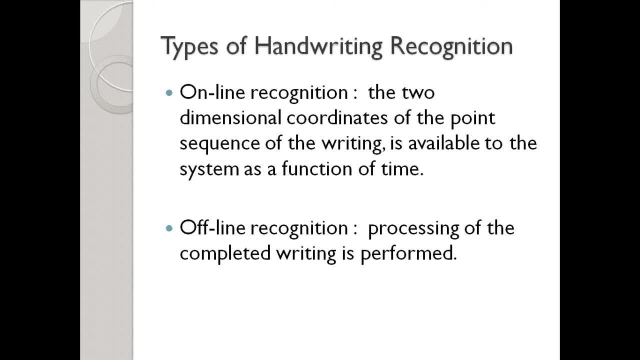 the two dimensional coordinates of the point sequence of the writing are available to the system as a function of time. Here pen tip movements are processed in real time to recognize the characters being written. On the other hand, in the offline type processing of the 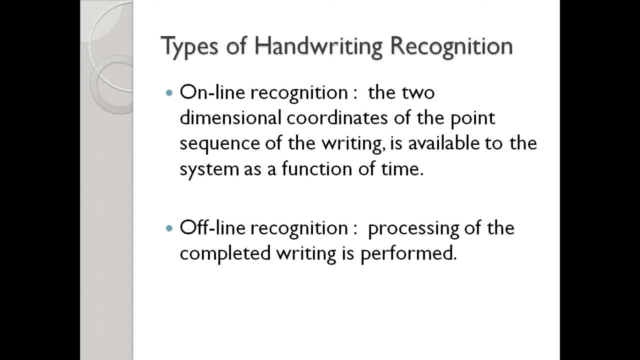 completed writing is instead performed. Offline handwriting recognition is indeed a difficult task, as different people have different handwritten styles. Narrowing the handwritten text to Narrowing down this problem domain to recognize handwritten digits from zero to nine would thus help to increase the accuracy of the recognition system. 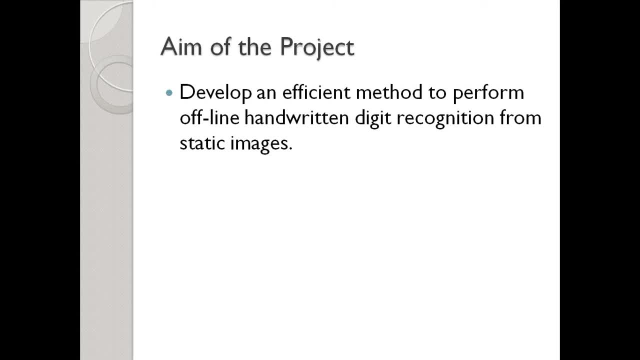 Hence the aim of my project is to develop an efficient method to perform offline handwritten digit recognition from static images. The process of offline handwritten digit recognition can be broken down into three stages. The first stage is to perform preprocessing of the input static image which has the handwritten 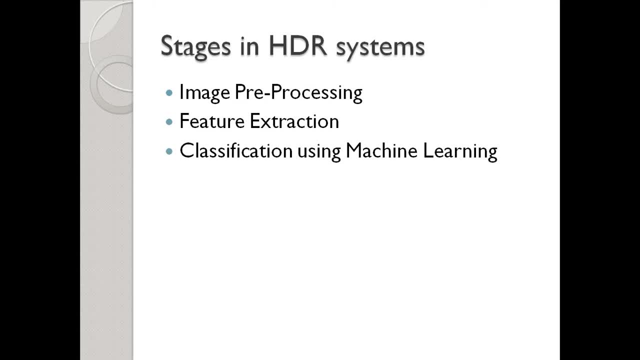 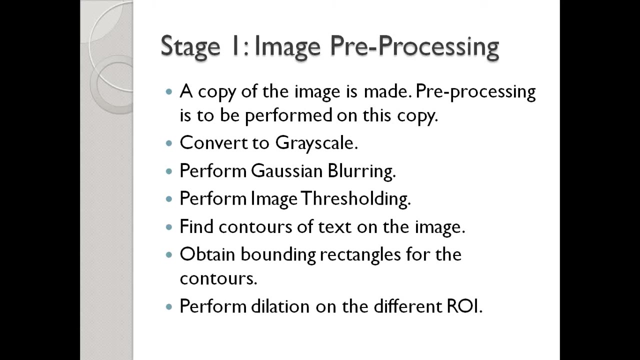 digits on them. obviously, This is done to identify the regions of interest on the image. The next stage is to extract the requisite features from these regions of interest. The last stage is to perform classification of the extracted digits. The input static image having the handwritten digits on it is preprocessed by using a sequence. 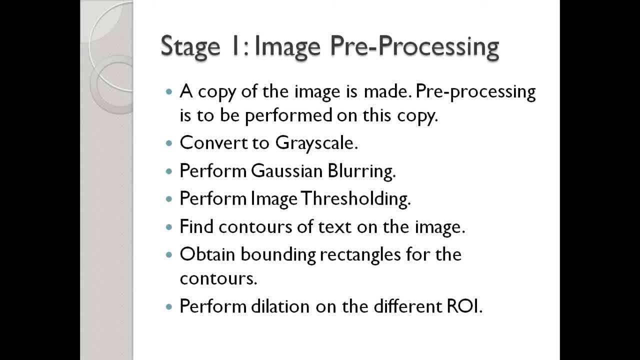 of steps, the regions of interest on that image. This process thus helps to identify the coordinates on the image where text is present. Initially, a copy of the image is made. Pre-processing is to be performed on this copy. Firstly, the copy is converted to grayscale Gaussian blurring is. 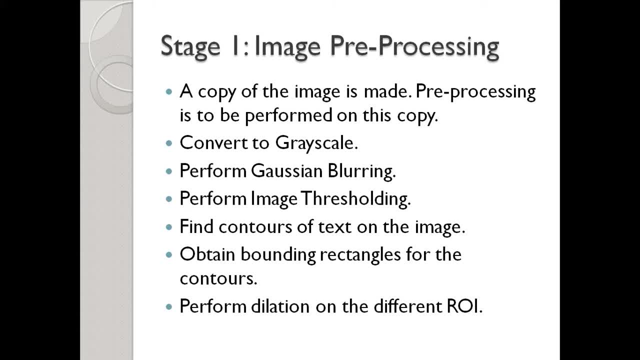 now performed to denoise and smooth this image Further. inverse thresholding is performed to convert the grayscale image to a binary image. Contours of the text, that is, the extreme contours on the image, are now found out. This is done by compressing the horizontal, vertical and diagonal. 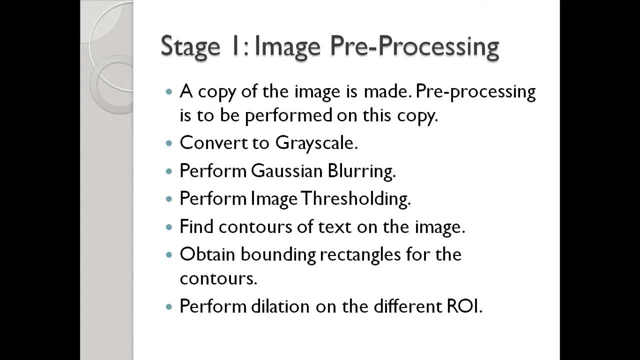 segments in the image to get their endpoints. Coordinates of the bounding rectangles for the various contours are then determined. The different regions of interest on the original image is a region within each of the bounding rectangles determined on the pre-processed image. Suitable dilation is further performed in these regions of interest on the pre-processed image. 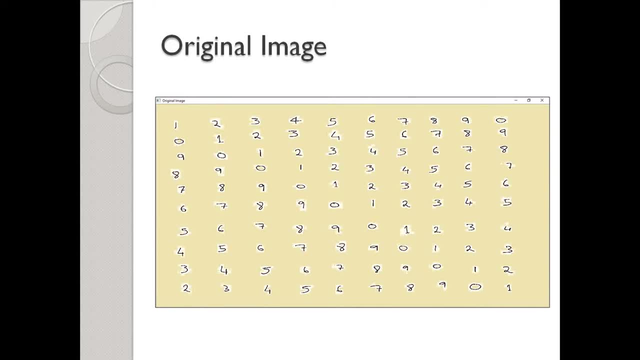 So this is an image I have used to test the image pre-processing- pre-processing: The first step of pre-processing is to convert the copy of the original image to grayscale. This is the grayscale image. Now the next step is to perform Gaussian Blurring. 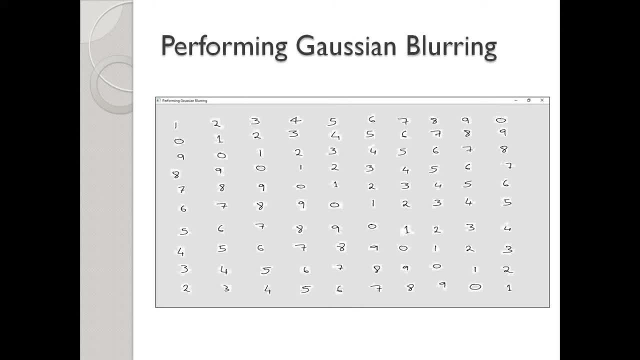 Essentially, what is being done in this step is blurring the image using a Gaussian function. As you can see, the image now becomes smooth. So I'm just taking the previous slide to see how the difference is. So if you focus on, say, any number like one over here, it does. 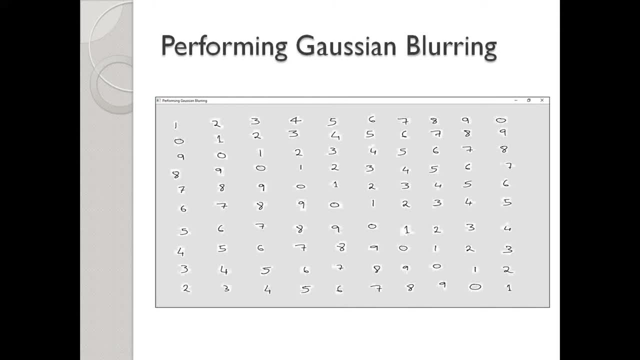 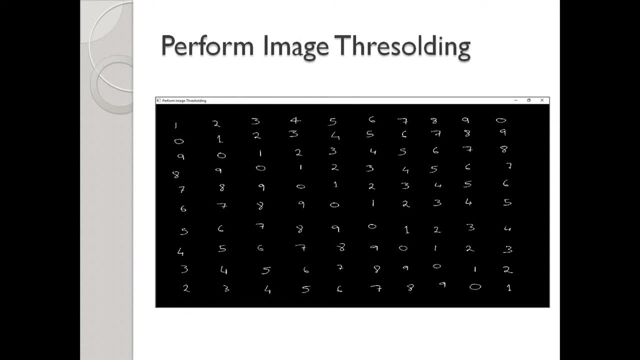 become smooth. The next step of image pre-processing is to perform image thresholding. Thresholding is the simplest method of image segmentation From the grayscale image. thresholding can be used to create a binary image. Here I'm using inverse thresholding to convert the 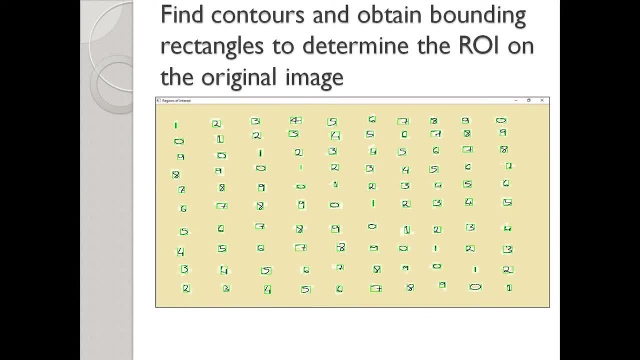 grayscale to a binary image. The next step in pre-processing is to find the contours of the text on the image. Coordinates of the bounding rectangle for the various contours are then determined. The different regions of interest on the original image is the region within each of the bounding. 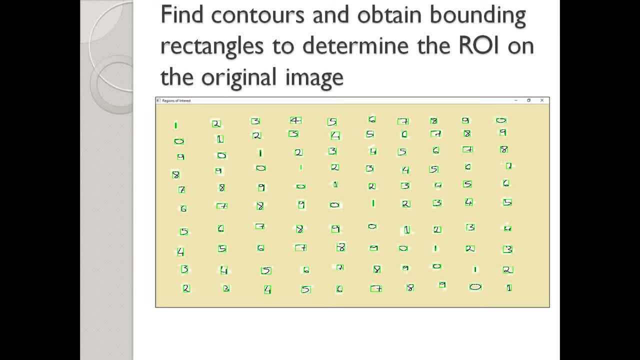 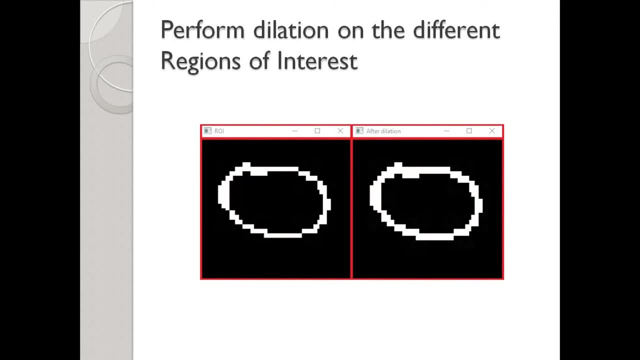 rectangles determined on the pre-processed image. As you can see, the various ROI have been marked on the original image using this technique As the final step in pre-processing dilation is performed. The dilation is to be performed on the various regions of interest on the image, which is 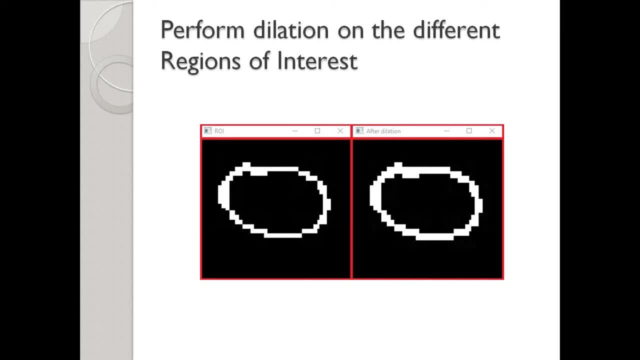 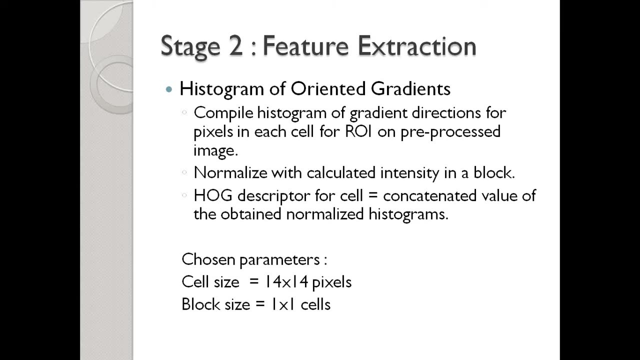 currently being pre-processed. This step essentially makes the object in white, that is, the inverse thresholded digits, bigger. The second major stage of handwritten digit recognition is feature extraction. I have used histogram of oriented gradients- feature extraction, for this purpose In this stage. 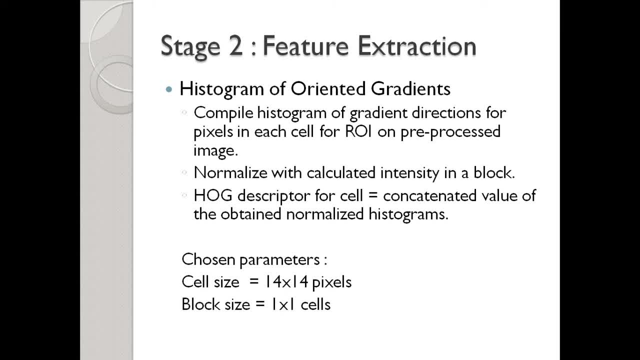 HOG feature calculation is performed for each of the rectangular regions of interest on the original image. HOG is essentially a feature descriptor that is used for the purpose of object detection in image processing and computer vision problems. The theory behind HOG is that any object within an image can be properly described by capturing. 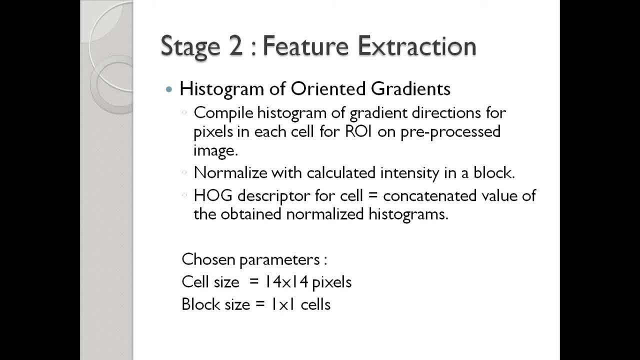 the distribution of intensity gradients. This is done by dividing the given image into small connected regions, called cells, and compiling the histogram of gradients for pixels within that cell. Usually these local histograms are normalized based on the calculated intensity over a larger region of the image. This is done by dividing the given image into small 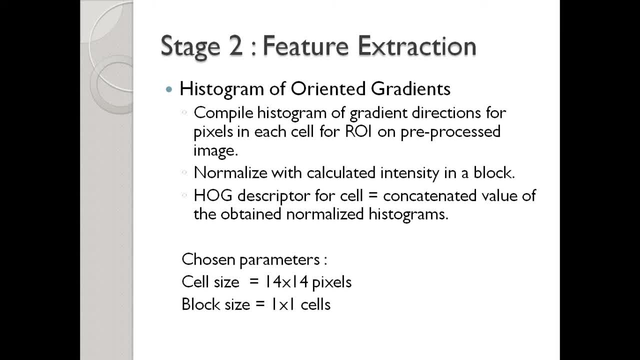 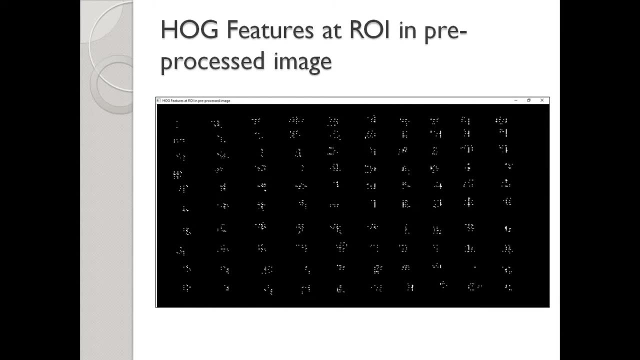 connected regions called blocks. The HOG descriptor for the cell is concatenation of the obtained normalized histograms. I have taken a cell size of 14 by 14 pixels and a block size of 1 by 1 cells in this project. This slide shows the HOG features in the different regions of interest in the image. 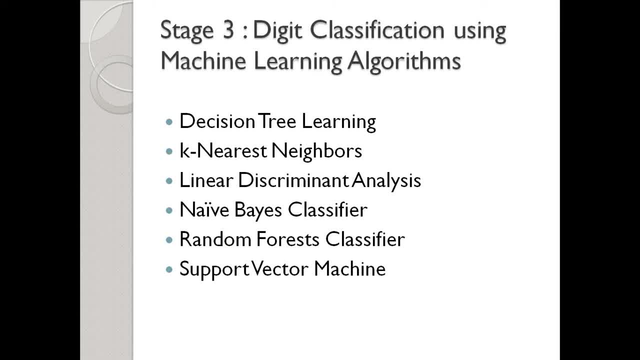 The next major task is to classify the digits as 0 to 9.. For this purpose, I have experimented with various machine learning algorithms. The ones that I have used in this project are: Dysentery Learning, K-Nearest Neighbors. Linear Discriminant Analysis. 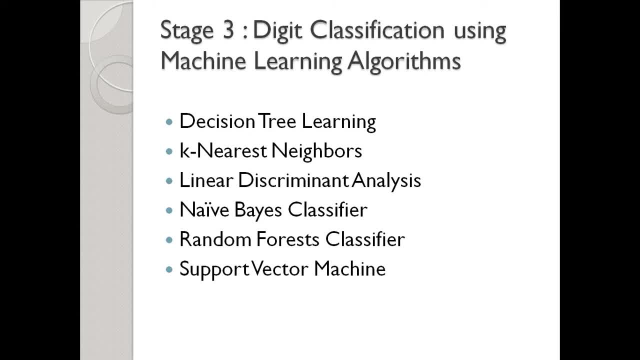 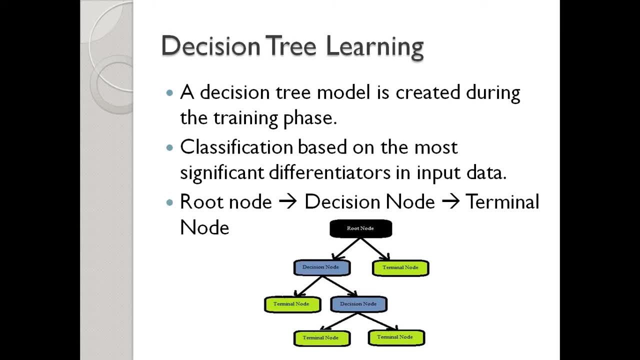 Naive Bayes Classifier, Random Forest Classifier and the Support Vector Machine. I'll give a brief description of each of these classifiers in the coming slides. Dysentery Learning: Dysentery Learning is a type of supervised learning algorithm. In this technique, a dysentery model is created during the training phase. 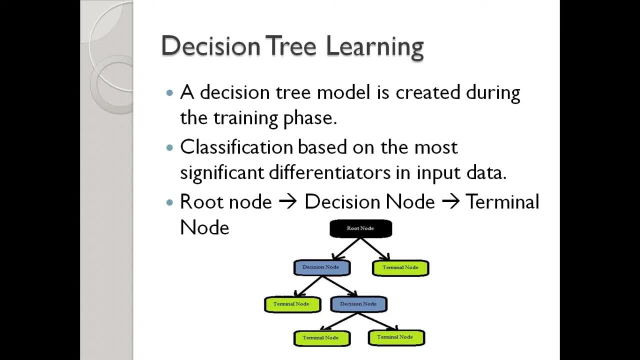 After training, any input to this model is then classified into one of the many subsets based on the most significant differentiators in that input. This is done by testing the input beginning from the root node to the different addition nodes. Ultimately, the terminal load will thus have the final result. 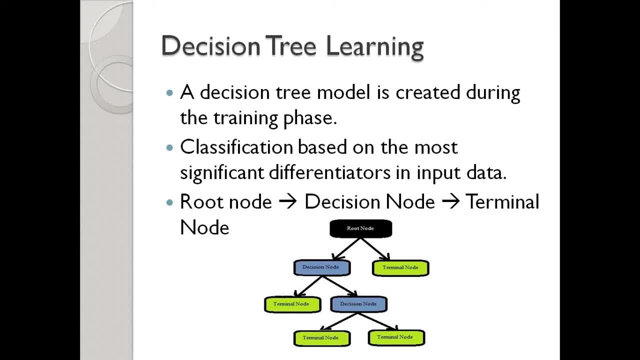 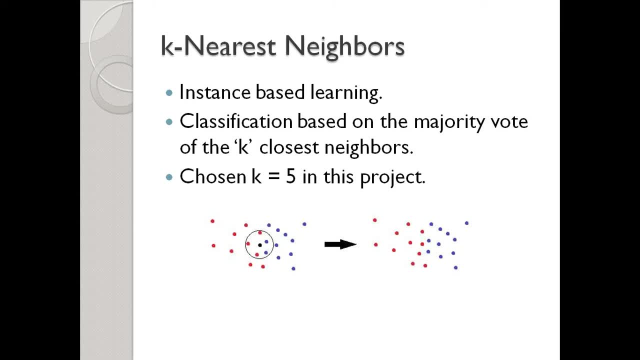 The advantage of Dysentery Learning is that it is easy to understand and is well suited for large data. K-Nearest Neighbors- K-Nearest Neighbors or KNN, is an instance-based learning technique. Here classification of an input data in the class is performed based on the majority word. 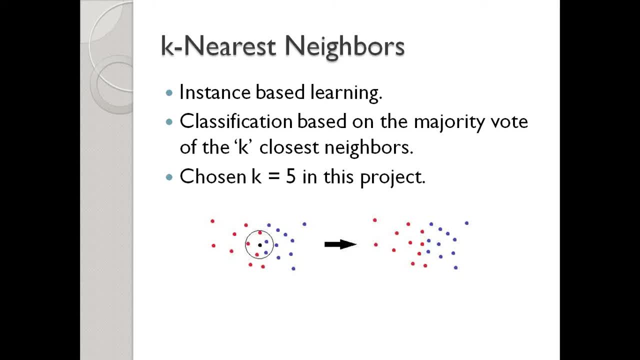 of the K-closest neighbors to this. given input, I have experimented with K equal to 5 in this project. The figure here represents an example of KNN with K equal to 5.. The unclassified data, that is, the black spot, is classified as a red spot. 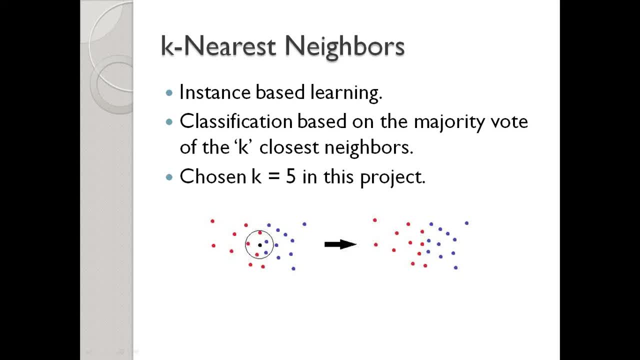 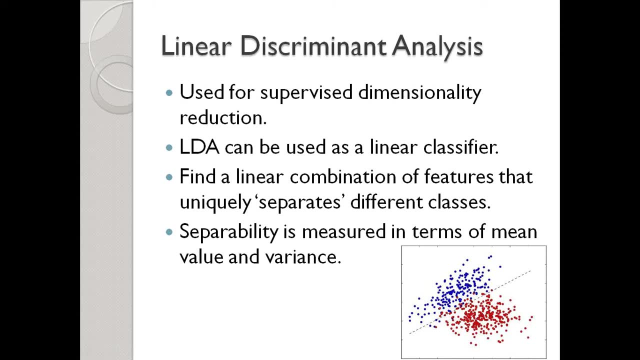 based on the words from the 5 of its closest neighbors. LDA- Linear Discriminant Analysis. LDA is a data analysis method generally used for supervised dimensionality reduction. LDA can be used as a linear classifier as well, by finding a linear combination of features. 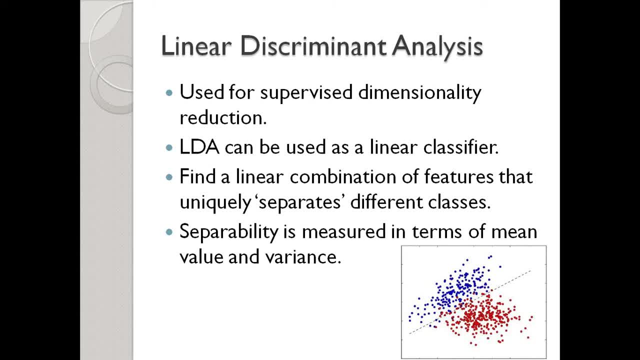 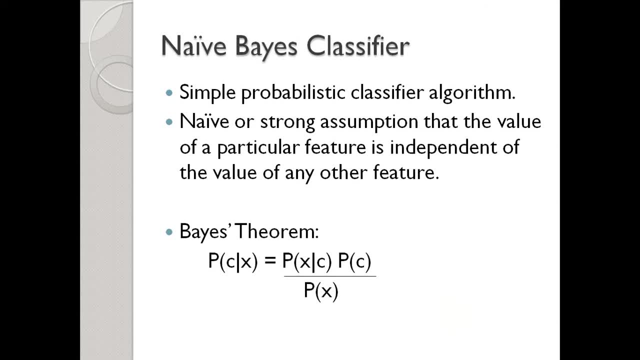 that uniquely separates different classes. This separability is measured in terms of mean value and the variance. The Naive Bayes Classifier. The Naive Bayes Classifier is a simple probabilistic classifier algorithm. It is based on the algorithm of the K-Nearest Neighbors. 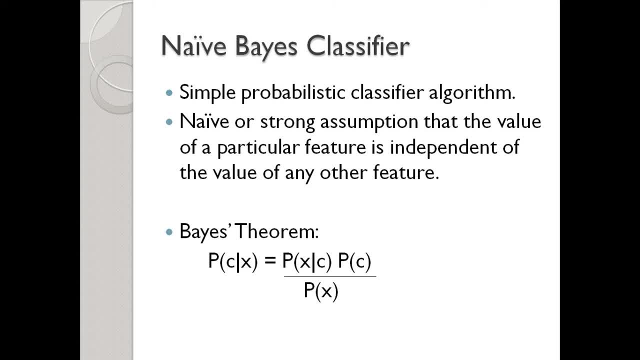 It is an application of the Bayes theorem with a naive or strong assumption that the value of a particular feature is independent of the value of any other feature. That is to say, this classifier considers each feature of an input data to contribute independently to the probability that the data belongs to a particular class. 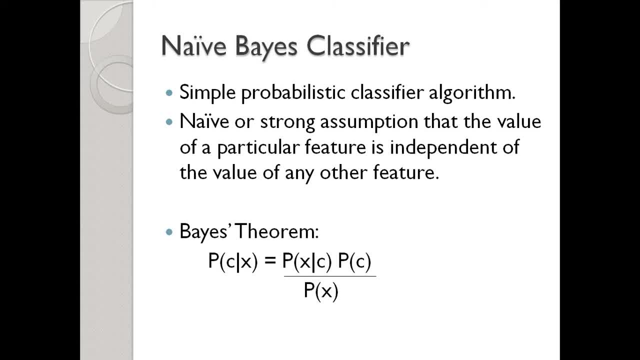 For example, a Naive Bayes classifier trained with a suitable dataset will classify a basketball as a basketball, independently considering its color, shape and diameter, regardless of any possible correlation between these attributes. The Bayes theorem used by this classifier is given here. 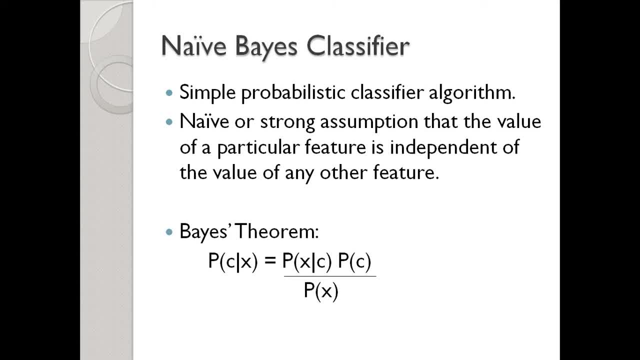 Here, Pc bar x is the posterior probability of the class given the predictor. P of c is the prior probability of the class. P x bar c is the likelihood and P of x is the prior probability of the predictor. On to Random Forest Classifier. 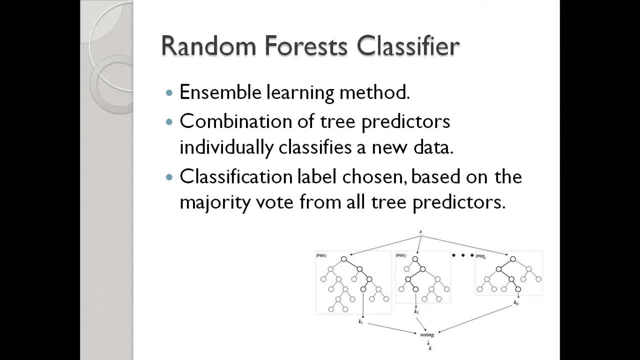 Now a random forest classifier is an ensemble learning method for classification. In this method, a number of distributions are calculated. A number of distant trees, together called a forest, are created during training. This combination of three predictors individually classifies a new data. 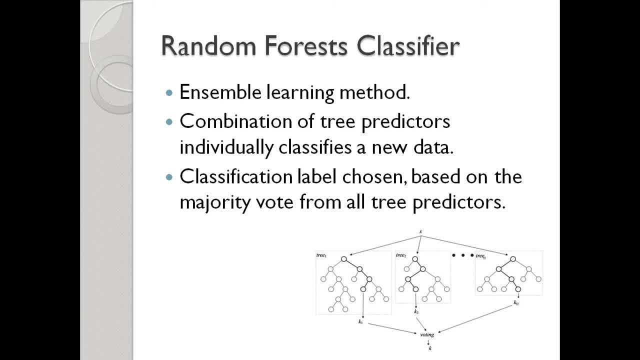 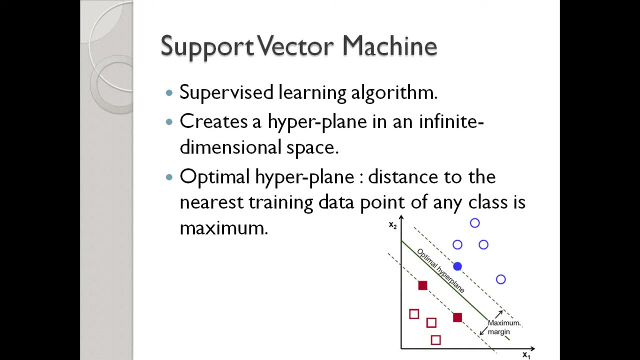 The forest chooses the classification label based on the majority word from all of these predictors. This makes a random forest classifier more robust than a single distant tree Support Vector Machine. Support Vector Machine, or SVM, is a supervised learning algorithm On training. an SVM classifier creates a hyperplane in an interval. 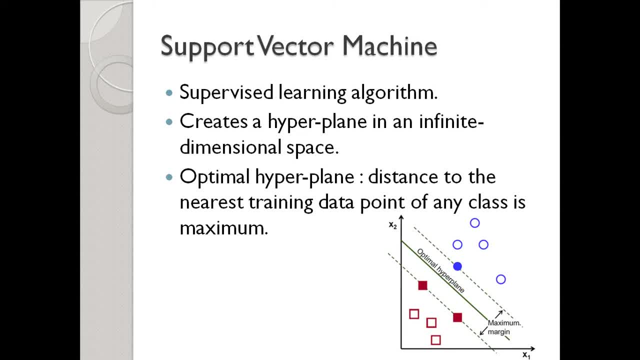 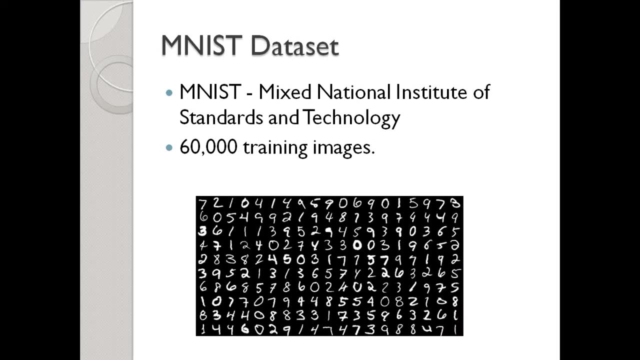 This is called a hyperplane. A hyperplane is set to be created when the distance to the nearest training data of any class is maximum. SVM makes use of the separating hyperplane to classify new data. All the recognition systems compared in this project made use of the same techniques for. 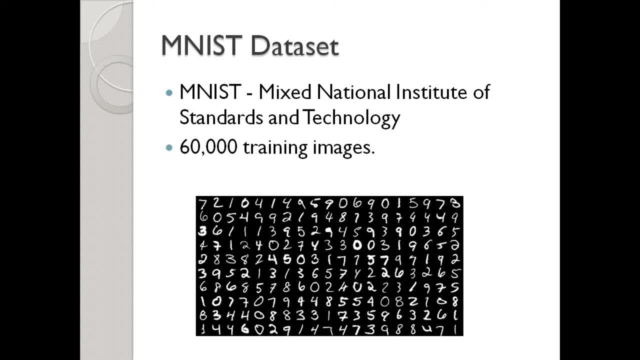